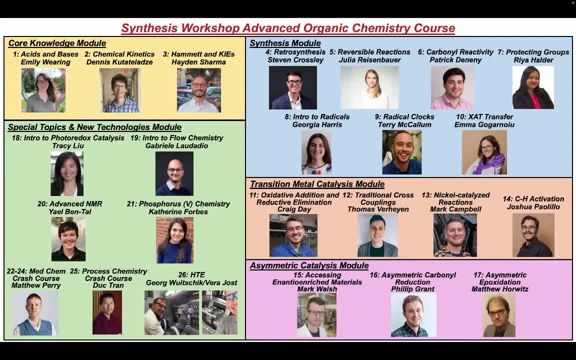 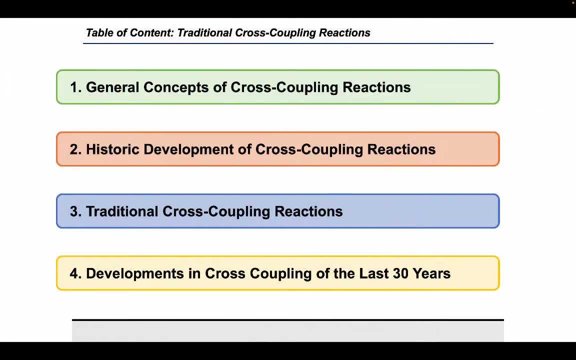 Thank you, Matt, for the introduction and the opportunity to again cut a tribute to this wonderful platform. Hello to everyone listening and welcome to today's episode of the Transition Metal Catalysis series in the Synthesis Workshop Advanced Organic Chemistry course. First we will have a look at transition metal catalyzed cross-couplings. 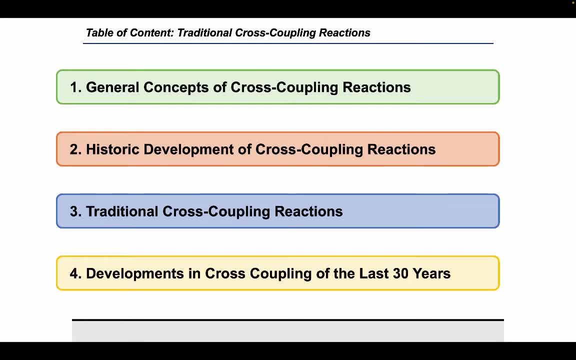 in general. Secondly, we will have a brief look at the origin of cross-coupling reactions. Next, we will look at the most popular cross-couplings and their related key publications. And finally, we will cover some key developments in the field of the past 30 years. 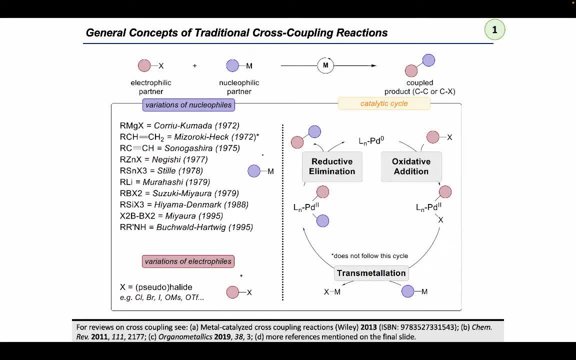 Metals have an important role in organic chemistry, especially in the field of cross-coupling. In essence, all cross-couplings discussed today, with exception of the Hecke reaction, can be simplified as a coupling of an electrophilic organoheate. 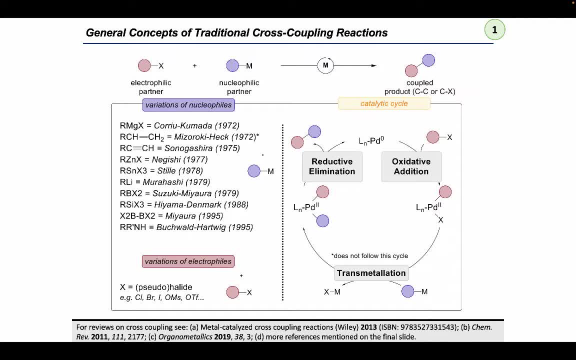 The Hecke reaction is a combination of a nucleophilic partner and a nucleophilic halide with a nucleophilic partner. Depending on the nucleophilic partners involved, different reactions have been developed over a 30-year span. In general, all the reactions in 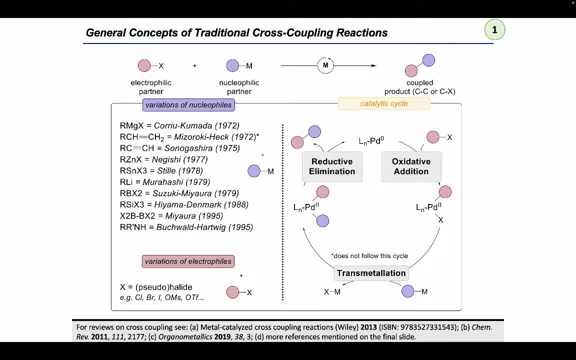 the list below follow the same simplified three-step mechanism, which is first oxidative addition, followed by transmethylation and finally reductive elimination to generate the final cross-coupling product. The individual steps are discussed in more detail in another episode. Related reactions will be discussed in a separate episode. 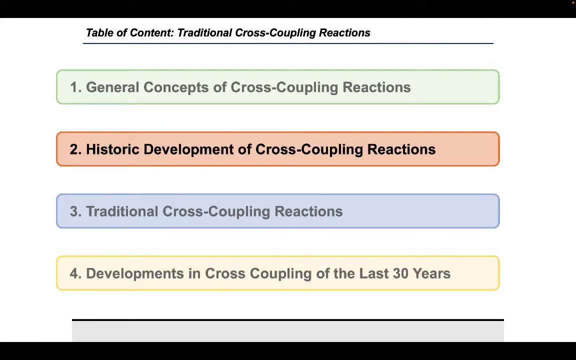 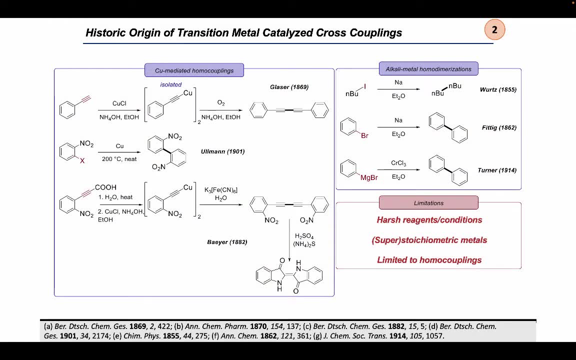 So where did transition metal-catalyzed cross-couplings come from? Critical to the development of cross-couplings are the stoichiometric metal-promoted homocouplings reported more than 150 years ago. For example, copper-mediated processes were developed early on in the groups of Glaser. 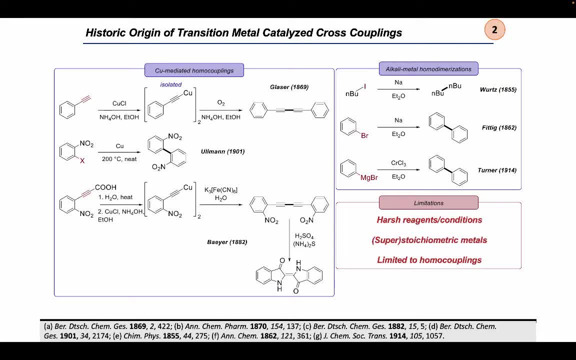 and Ullmann. While both rely on stoichiometric copper, the Ullmann methodology is different, since a carbon-halogen bond rather than an unfunctionalized carbon system was used in the dimerization. The synthetic potential of the copper-catalyzed homodimerization developed by Glaser. 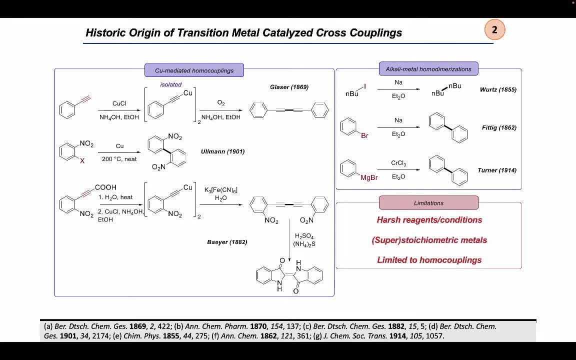 was, for example, demonstrated in the industrial synthesis of Indigo by Bayer. Even earlier, the ferocious reactivity of sodium and potassium alkali metal reagents was exploited in the homodimerization by the groups of Wurz and Fitt. Of course, the high reactivity of both reagents 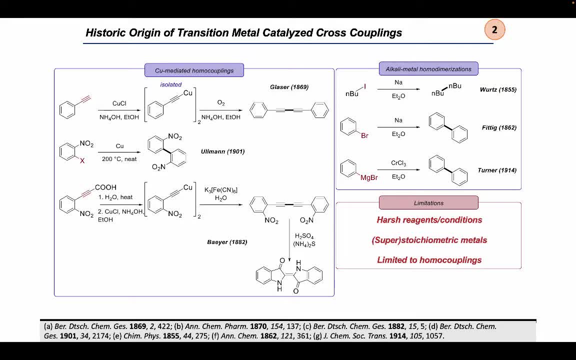 strongly limited the potential of the homodimerization of the copper-catalyzed homodimerization. So the first to use Grignard's reagents in a coupling reaction was Turner, who reported the dimerization of these reagents mediated by initially chromium and a few years later by copper. 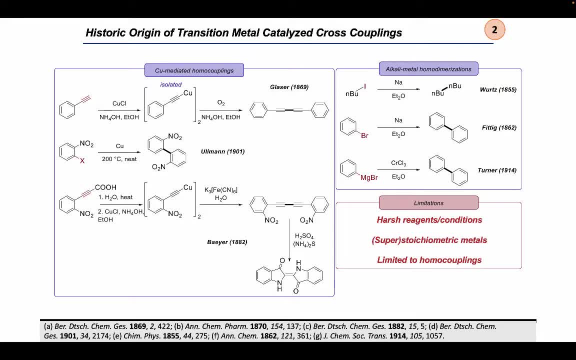 Moving away from the harsh reactivity of alkali metal reagents to Grignard's reagents is a significant improvement, but all the processes shown here rely on harsh conditions, stoichiometric or super-stoichiometric metal reagents, and the transformations are limited to. 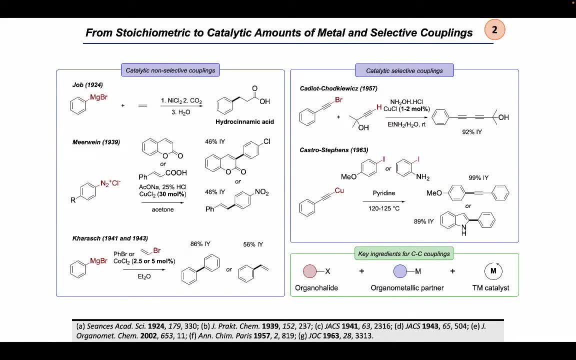 the normal couplings. The first use of catalytic rather than stoichiometric amounts of metal can be traced back to the work of Job Merouin and Karrasch, Job far ahead of his time, reported in 1924. 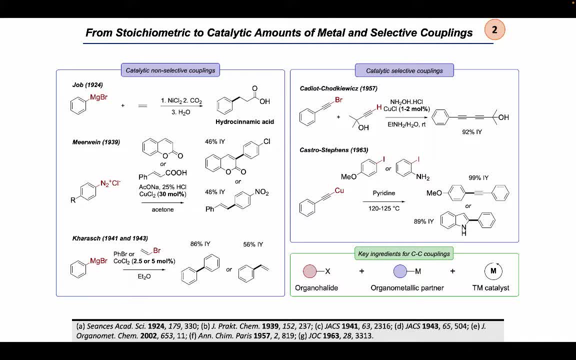 that phenylmagnesium bromide in the presence of nickel chloride generated a derivative able to react with various gases such as ethylene, carbon monoxide and hydrogen. In the example shown published one year later, he successfully isolated hydrocinnamic acid and demonstrated: 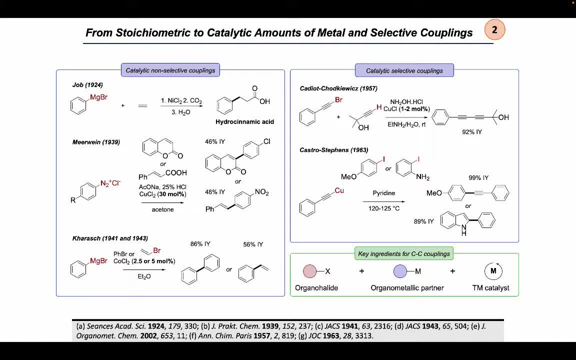 that the reaction outcome with a fixed amount of ethylene was independent of the amount of nickel used. The work by Merouin in 1939 on copper-catalyzed coupling of aryldiazonium salts with alkenes, leading to coumarins and cinnamic acids, is also an early example of catalytic metal use. 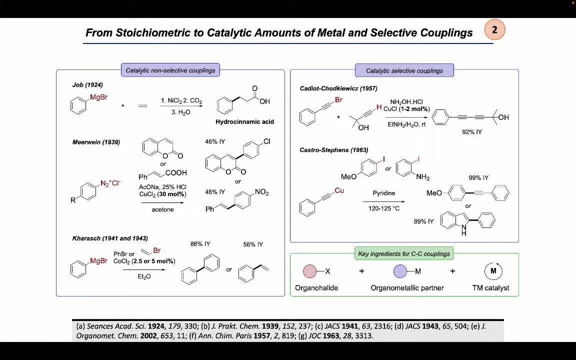 However, neither of the two contributions was picked up by the scientific community. In contrast, the work of Karrasch was picked up by the scientific community, maybe because he provided a systematic and more detailed investigation of carbon-carbon couplings in a series of publications starting. 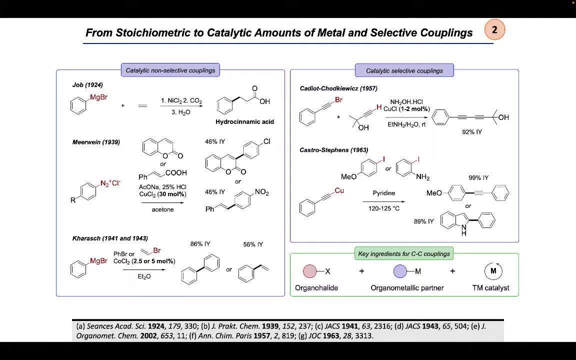 with the first publication in 1941.. The key breakthrough report was published two years later, in which he described the cobalt-catalyzed cross coupling of phenyl bromide with aryl magnesium bromide. This represents the earliest detailed report of a cross coupling rather than a homocoupling. 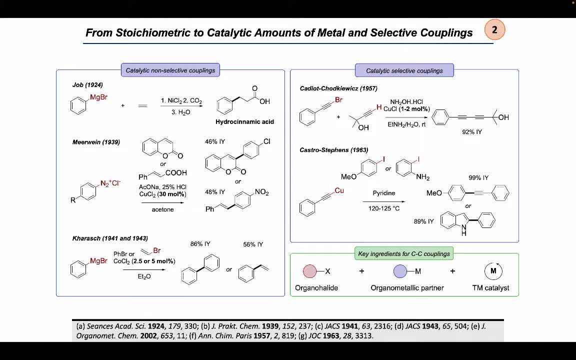 and thus Karrasch can be considered as the grandfather of carbon-carbon couplings. Starting from this point, multiple groups got involved, and especially the subsequent work of Gauthier and co-workers on the mechanism should be highlighted, since it helped to further understand. 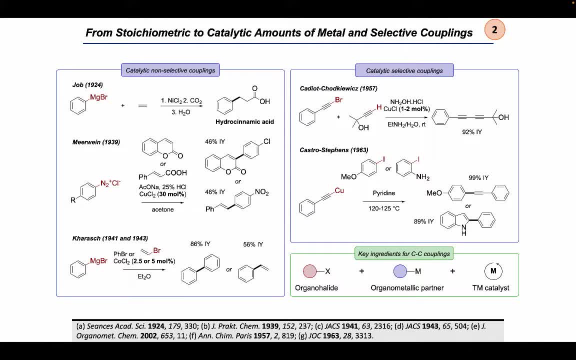 and develop the field of cross-couplings. Several years later, also the first catalytic copper-carbon carbon bond formation reactions were reported by Cadell-Czoskiewicz and Castro-Stevens. These examples represent a breakthrough because they provide a desired product with high selectivity, avoiding 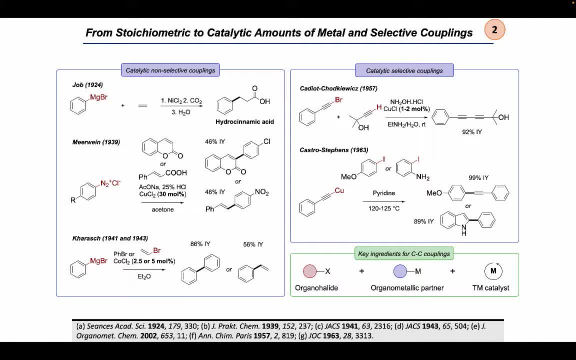 the undesired competing homogenization. All the combined contributions shown on this slide demonstrate for the first time the use of catalytic rather than stoichiometric quantities of transition metal to form the desired carbon-carbon bond. Secondly, they provide the first selective cross coupling and, based on these reports, 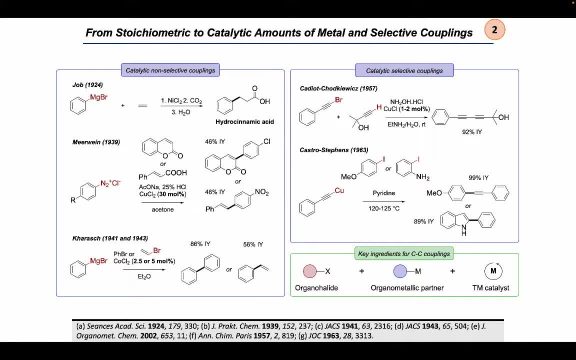 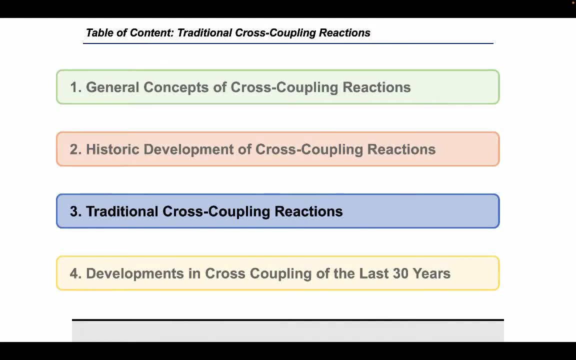 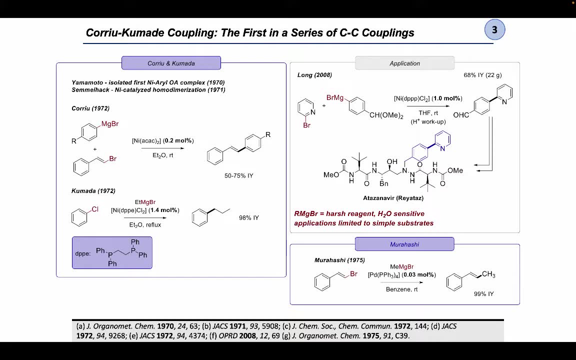 the three key ingredients for a successful cross coupling were identified. Now we will have a look at several important cross couplings and their initial reports. After the detailed work of Kares, the scientific community became aware of the potential of cross couplings and more people became involved, leading to further improvements. A major milestone was 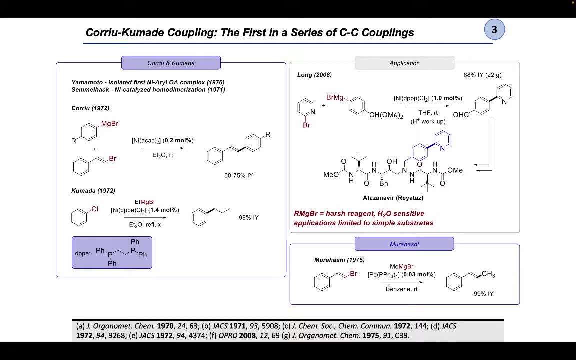 reported independently by both Coriou and Kumada and co-workers. Both introduced nickel as a transition metal in the cross coupling of organo-magnesium partners. The idea to introduce nickel was based on previous work by Yamamoto, who had successfully isolated the first nickel-aryl-halide. 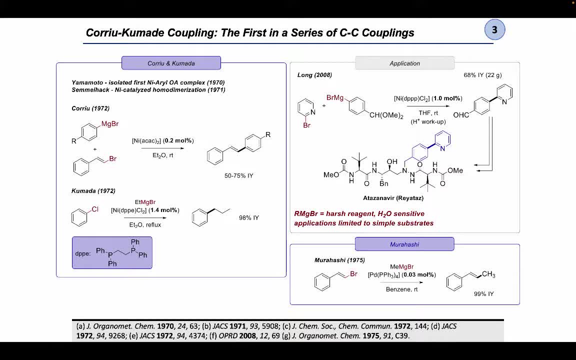 oxidate-fedition complex and Semmelheck's related work on the nickel-catalyzed homodimerization. Apart from the selective cross coupling, also the introduction of a phosphine ligand by Kumada are noteworthy breakthroughs in the field. The Coriou-Kumada coupling was, for example, applied. 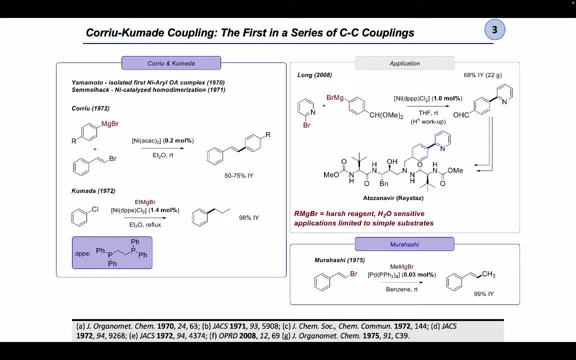 in the synthesis of an early bioaryl intermediate of the HIV protease inhibitor, atazanivir. Despite its novel approach to construct carbon-carbon bonds, the high reactivity of the organo-magnesium compound is a significant improvement in the process. 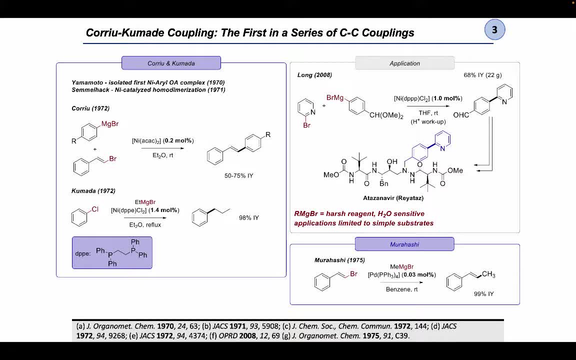 It is the major limitation of this methodology, since they react with a variety of electrophiles and are also sensitive to water. The Kumada coupling can also be catalyzed by palladium instead of copper. The palladium-catalyzed variant was first reported by the group of Murahashi. 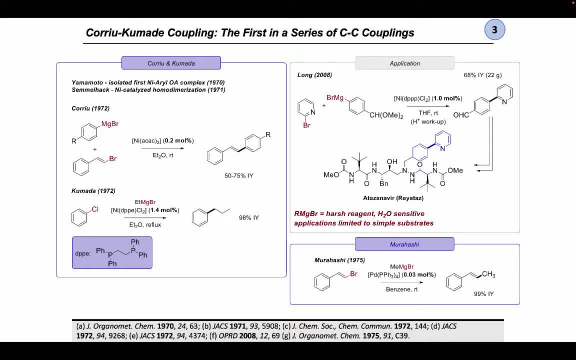 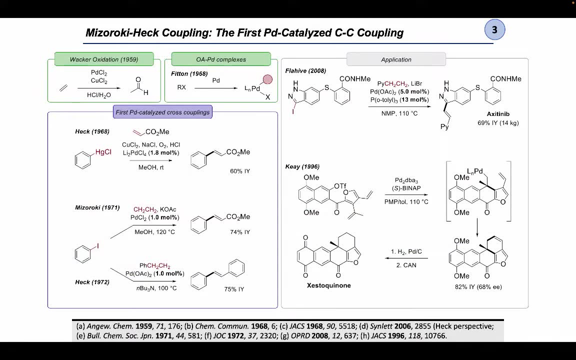 Tetrakis. triphenylphosphine palladium, or also often referred to as tetrakis, is used as both palladium source and ligand. The idea of using palladium in the Kumada coupling can be attributed to a series of publications in 1968, with Hegg as sole author In these. Hegg describes the coupling. 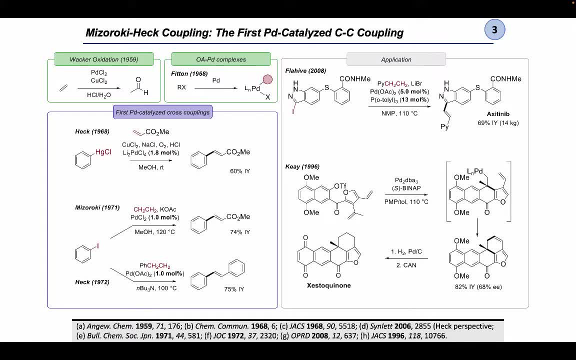 of organo-mercury reagents with various alkenes catalyzed by palladium. One of his earliest examples is shown on the slide. Most likely Hegg was inspired to use palladium based on its prior use in the Wacker oxidation. Improvements were made in the following years by both Hegg and 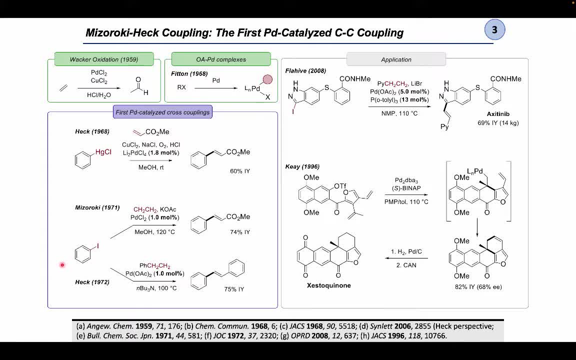 Mizoroki, who were the first to use palladium in the Kumada coupling In the early 2000s, for example, as shown by replacing the toxic organo-mercury reagents by organohalides inspired by earlier work of Phyton on the oxidative addition products of palladium and organohalides. 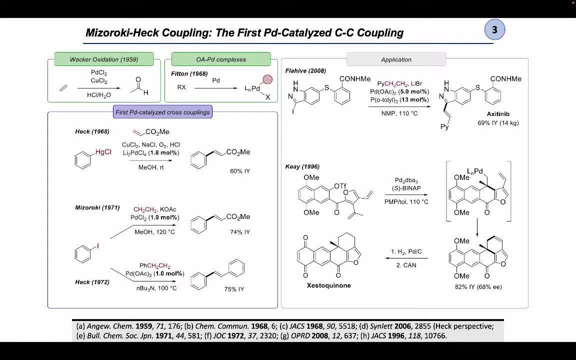 The Mizoroki-Hegg reaction has become a popular method in the arsenal of synthetic chemists due to its broad functional group tolerance, but of course it requires an alkene. A large-scale application of this methodology was reported by Flyheave and co-workers at Pfizer. in the final step, 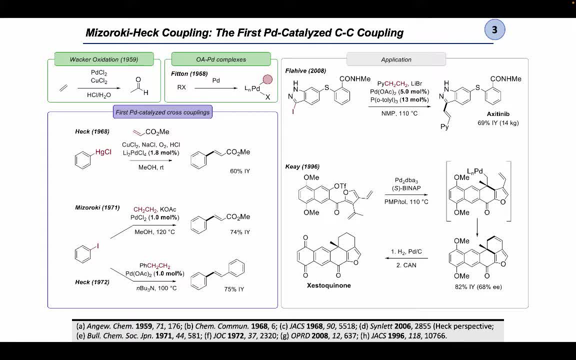 of the development of a new method for the treatment of cancer. Another very nice example of a cascade: double-Hegg asymmetric cyclization was demonstrated by Key and co-workers as a crucial step in the total synthesis of xestylquinone. From this point on, palladium would be a transition. 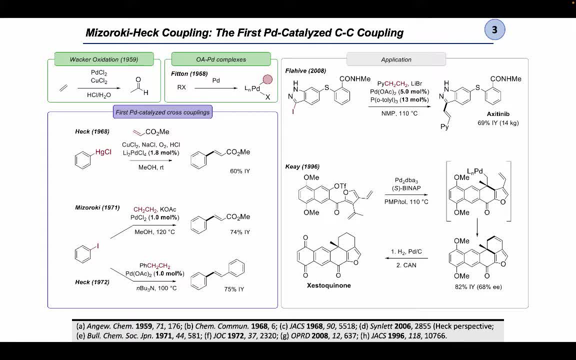 metal to consider for future applications, apart from copper and nickel, who had dominated the landscape thus far. Over the years, the scope of palladium in cross-couplings, as you will see in the next slides, would grow, and often palladium would argue with the use of palladium in the process. 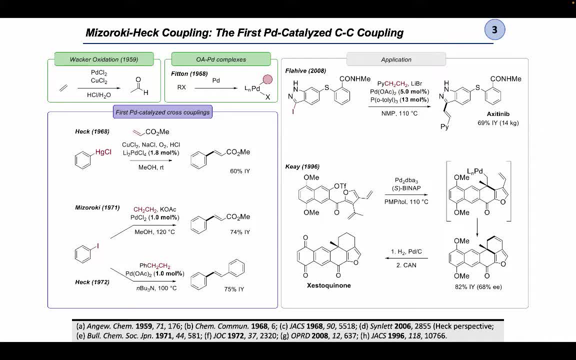 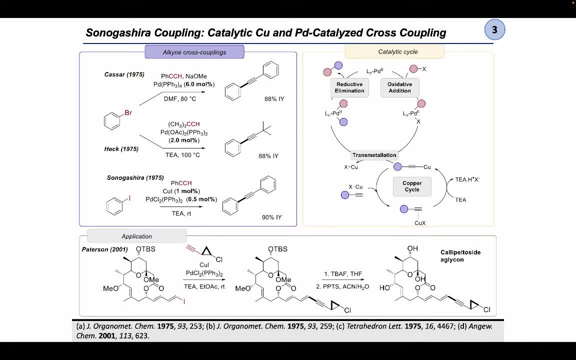 For example, in the field of acetylene couplings, copper salts were the catalyst of choice early on. However, this changed, as in 1975, three groups- Casar-Hegg and Sonegashira- independently described the first palladium-catalyzed coupling of acetylenes with aryl and phenyl halides. 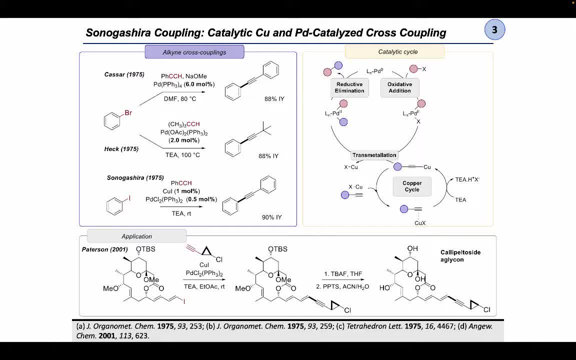 We observe that the combination of copper with palladium by Sonegashira allows much milder conditions versus the conditions of palladium-catalyzed copper-acetylene-acetylene-acetylene With only palladium of Casar and Hegg. most likely, the base and copper result in the formation of a 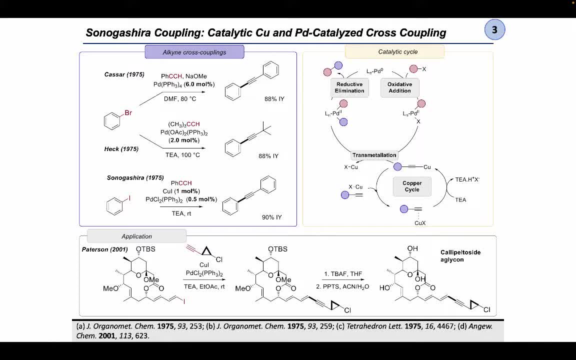 copper acetylide, which accelerates the transmethylation step. The combination of palladium and copper developed by Sonegashira is still used in modern applications. For example, in the 20-step total synthesis shown on the slide, a late-stage Sonegashira coupling is used. 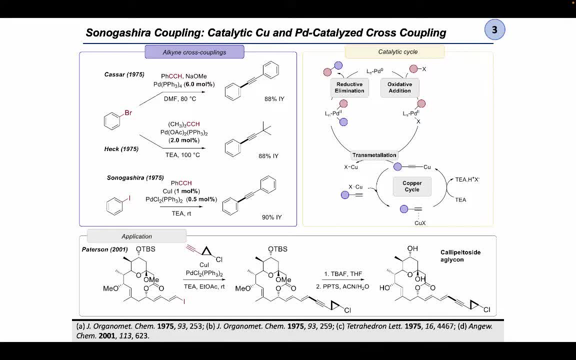 The mild conditions leading to a high functional group tolerance, combined with the availability of acetylenes and aryl halides, places the Sonegashira method in an excellent position for both early and late-stage modifications. Of course, the need of acetylenes also limits the product. 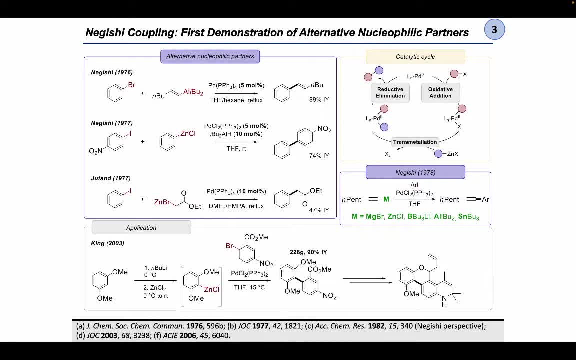 diversity. An important milestone in the field of cross-couplings was reported in the 1970s by Nekishi. Less reactive organometallic reagents such as organoaluminium and organozinc reagents were introduced by Nekishi. Also, Jutton reported the use of organozinc reagents. 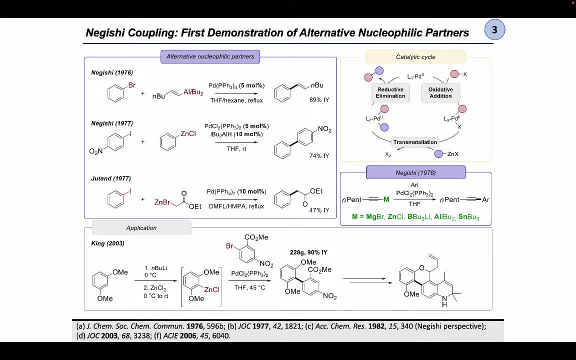 in cross-coupling. around the same time, Further studies on the coupling itself, mostly by Nekishi but also by other groups, and studies to generate zinc species by, for example, the Knochel and Ukiyama group, have resulted in a broad scope and thus made. 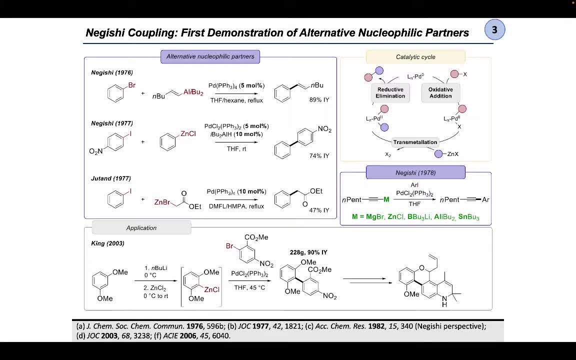 this an essential reaction for the synthetic chemists, especially in the field of total synthesis. An example of the Nekishi reaction in industry was reported by chemists at Abbott. The zinc species was made by litigation, followed by the slow addition of the zinc source. Next the aryl bromide and palladium ligand were added to obtain the 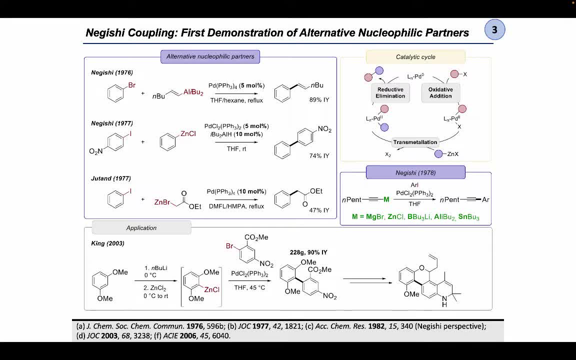 desired intermediate on large scale. Also, no theaster functionality on the intermediate, which would not be compatible with an organomagnesium reagent. The major downside is the operational complexity and waste of the zinc species, which explain its overall limited use in industry, Most importantly, having demonstrated the reactivity of alternative. 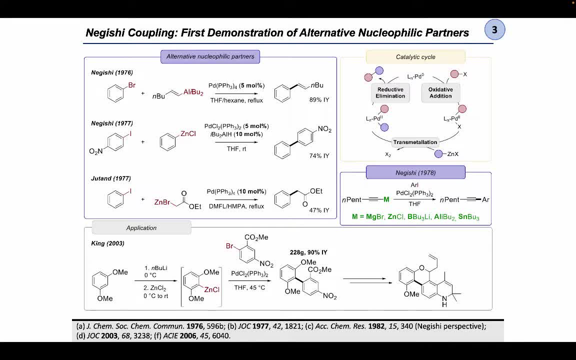 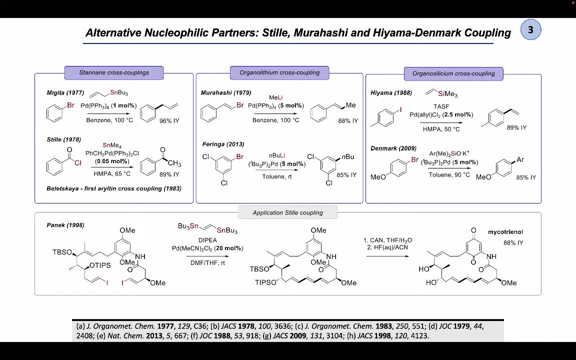 organometallic derivatives instead of organomagnesium, Nekishi set a stage for the uncovering of milder, less electropositive metal coupling species. Other alternative organometallic derivatives followed shortly after the pioneering work of Nekishi. Two key contributions from Stille and Migita on the selective coupling of 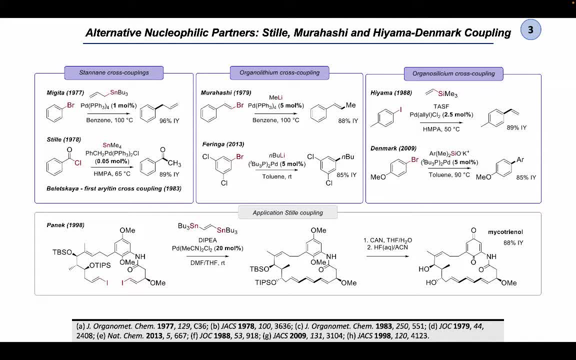 organostannanes are shown with pioneering work by Eborn Atwell, Boeckermann and Matsumato paved the way. Also, the expansion from alkyltin to aylotin reactions by the biletskaia is an important contribution to the field. Stille and his students further optimized. 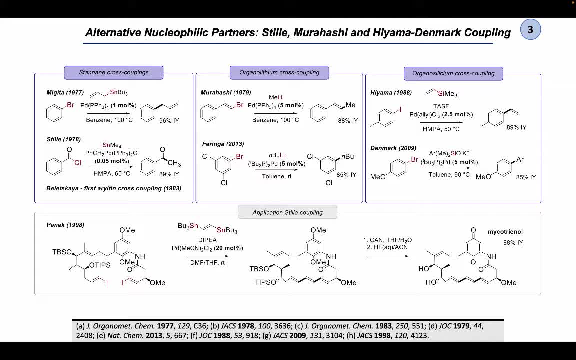 the cross-coupling of stannanes with organohalines. The Stille coupling can be used in the synthesis of complex compounds, For example in the synthesis of mycotrinol, the late-stage tandem Stille-microcyclic. 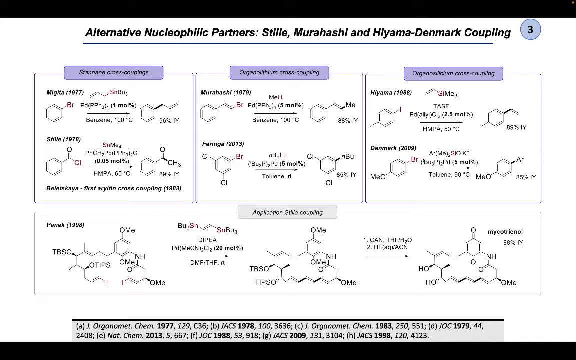 coupling is followed by oxidation and deprotection to produce the desired natural product. The introduction of organolithium species can be traced back to a report of Murahashi and co-workers. The Murahashi coupling is less known due to the strong reactivity. 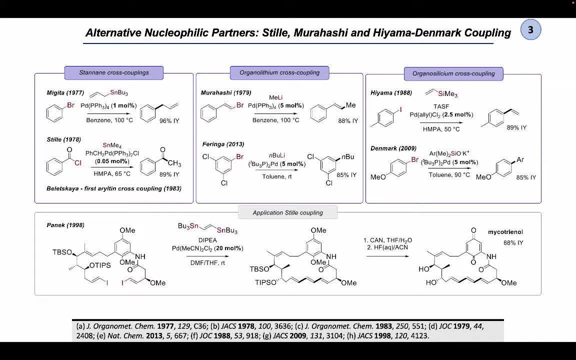 and difficult handling of organolithium reagents. Recent development shown by the example of the Ferrignier group have improved reaction conditions by using modern catalytic systems and appropriate conditions. The major advantage is the low cost and availability of the lithium reagents, but the functional group tolerance remains a challenge even today. Another 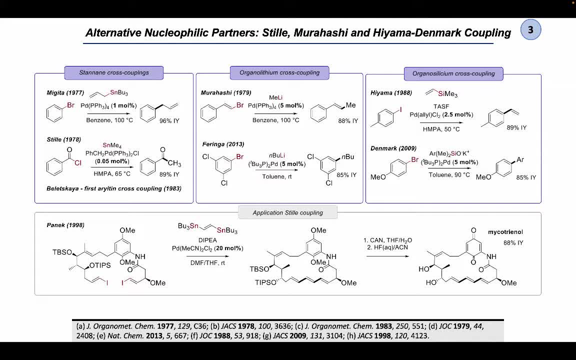 alternative organometallic discovered later are silanes, which can be linked to the work of Hiyama and co-workers. The first report in 1988, by Hiyama, shows that the inclusion of a fluorine source, thus in this case in the reaction mixture. 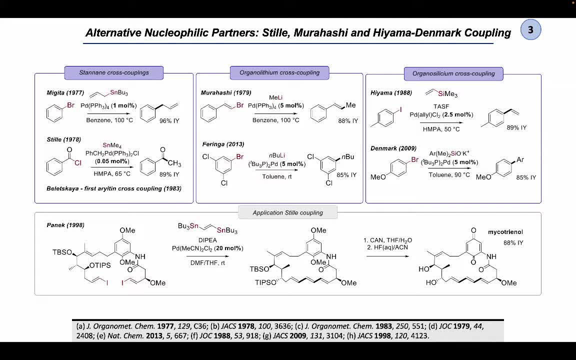 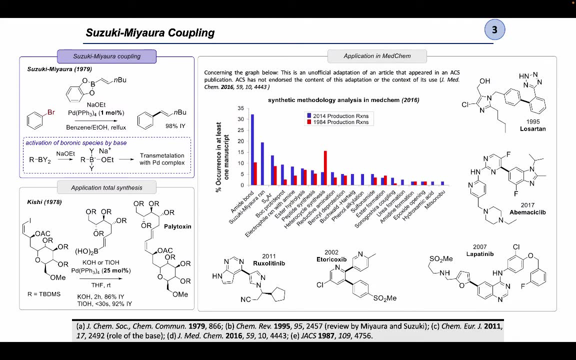 can be used to activate the organosilane towards transmethylation. This methodology was expanded by the group of Denmark, For example by using other silane reagents. a bronze set base instead of a fluorine source could be used for the activation. The most known and used 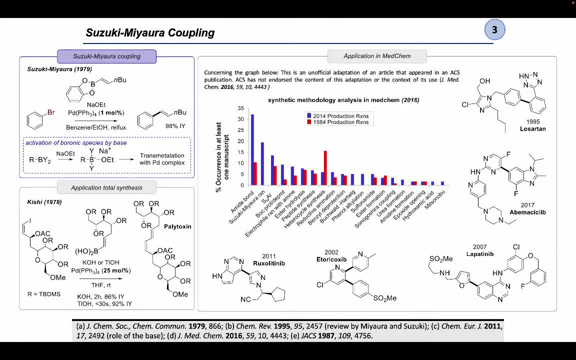 organometallic coupling partner and related cross-coupling are boronic species used in Suzuki-Maiora cross-coupling. The first catalytic cross-coupling of boronic species can be linked to a report by Maiora and Suzuki in 1979, based on earlier similar but non-catalytic coupling data. 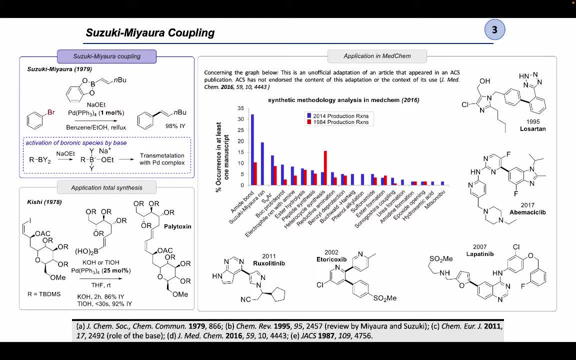 of both Negishi and Heck. The versatile adaption by both academia and industry of this carbon-carbon bond-forming strap G can be understood by the boron coupling partner which, contrary to previous couplings- easy handling, air and moisture stability- is less toxic and has more easily removed less toxic. 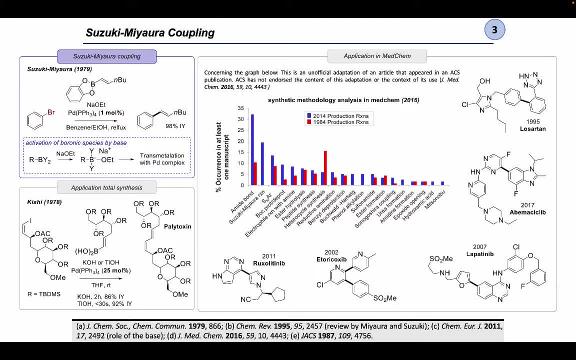 byproducts. It's also important to note that the base plays multiple roles, such as the activation of the boronic species, and thus is required for the reaction. The number of examples of Suzuki Miura couplings in the pharmaceutical industry are vast. An analysis published in 2016 of past 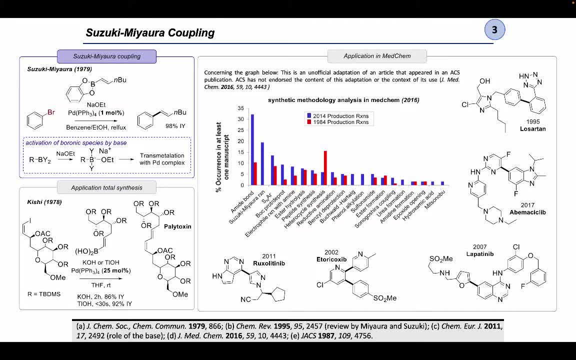 and present synthetic methodologies applied in medicinal chemistry shows that three couplings are used frequently. These are Sonogashira, discussed before, the Buchwald-Eftrich coupling to be discussed, but most heavily used of the three is the Suzuki Miura coupling. In fact. 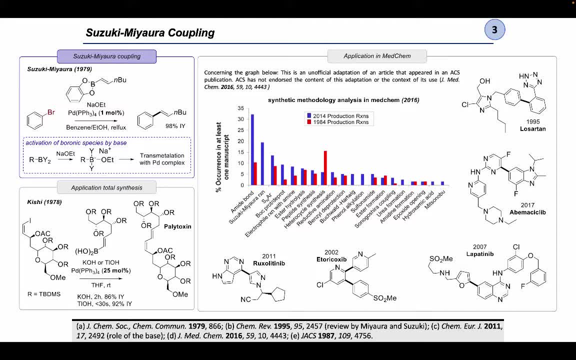 Suzuki Miura. cross-coupling is in the top five most frequently occurring reactions. Examples of biphenyls prepared via this coupling in proof drugs are often observed, as you can see by the examples. A second early example in the total synthesis of palytoxin was reported by Kishi. 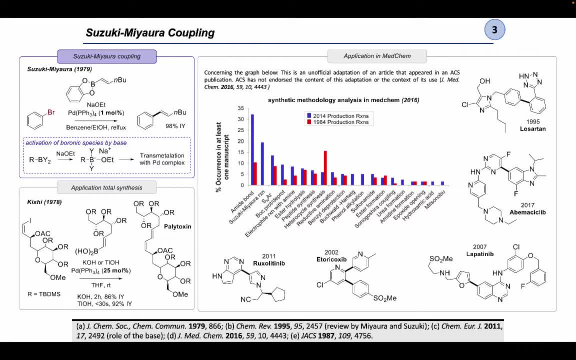 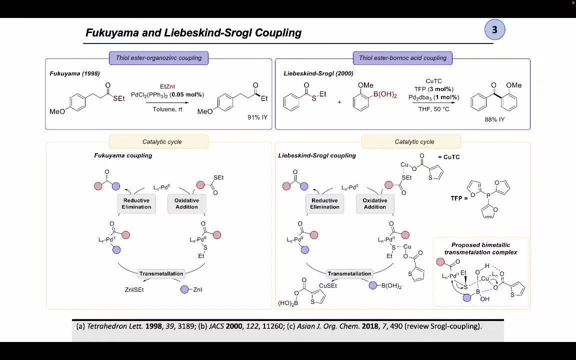 and Hyaluronic Acid. Kishi highlights the importance of base Use of thalium hydroxide gives complete reaction upon mixing of the reagents, while potassium hydroxide requires two hours to reach high and yet incomplete conversion. To complete the carbon-carbon-pladium-catalyzed cross-couplings, we must also mention two. 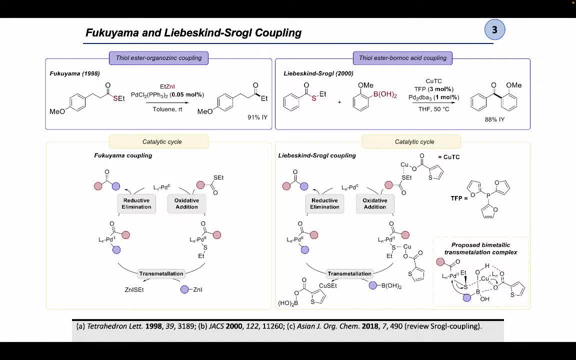 more related couplings developed in the late 1990s. Both lead to ketone products and both make use of a thioester as a coupling partner. First, the Fukuyama coupling is a plate used to make a cross-coupling with an organo-zinc halide and a thioester. The reactivity and the mechanism. 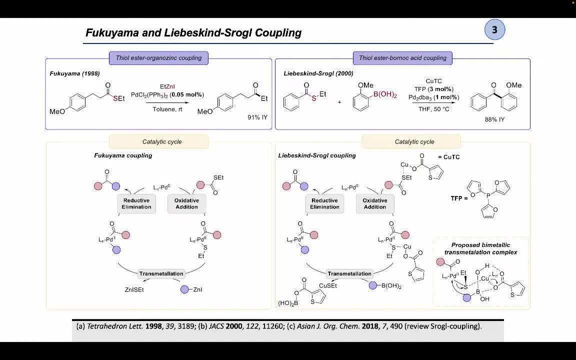 are like the Nogishi coupling, where the thioester is used instead of an organo-halide as cross-coupling partner. Again, due to the use of the zinc reagent, the coupling can be done under mild conditions. 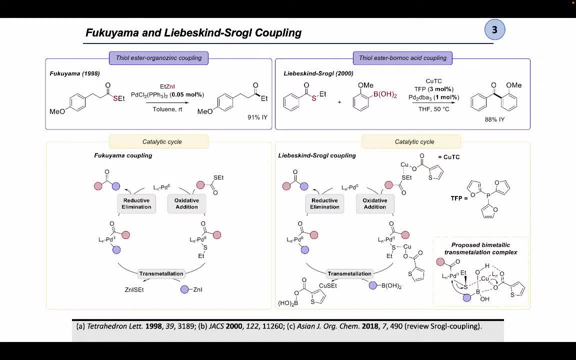 thus has a broad functional group compatibility, but also results in operational complexity and large amounts of zinc waste. A final noteworthy addition to the carbon-carbon cross-coupling toolbox is the Kishi-Kamikaze coupling. The Kishi-Kamikaze coupling is a 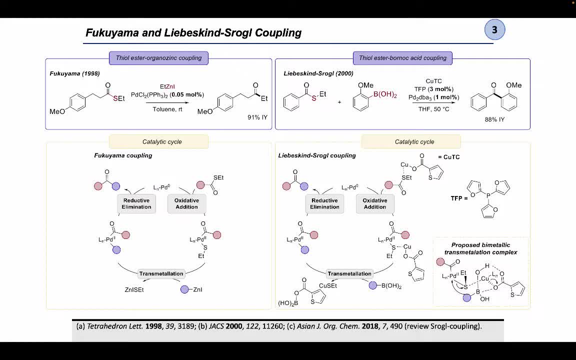 carbon-carbon bond formed from a thioester and a boronic acid, using palladium as catalysts and stoichiometric amounts of copper. The critical transmethylation step is proposed to go via a copper and palladium bimetallic complex, with all the coupling partners present Apart from thioesters. 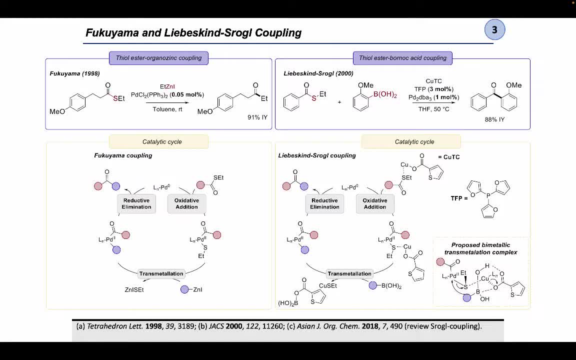 also thioethers, thioamides, thioalkynes and thioisocyanides have been used as electrophiles Also. the Nucleotide-Coupling Toolbox is the Liebeskind-Schuh coupling In the original report. 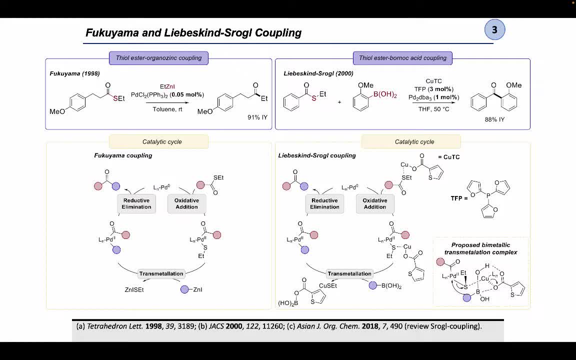 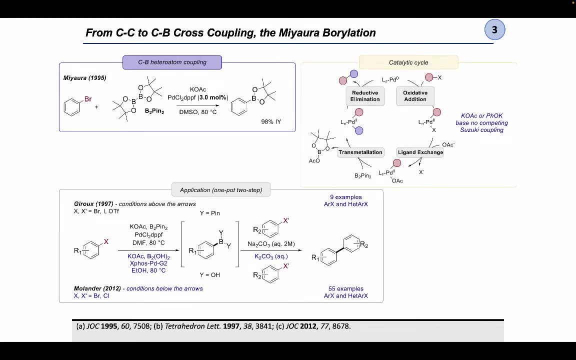 the Nucleophilic-Boronic-Asset partner can be changed to, for example, stannanes, indanes and others. Variants catalytic in both palladium and copper have also been developed after the initial report. A challenge which remained unaddressed is the cross-coupling of non-carbon nucleophiles. 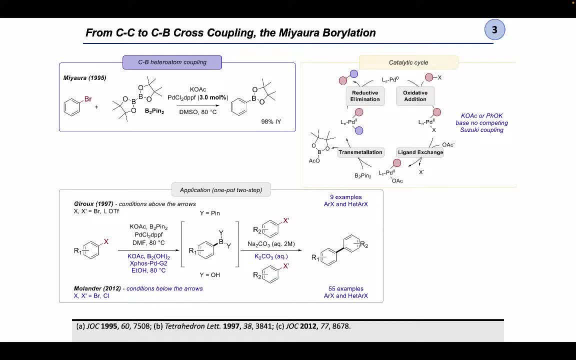 to form carbon-heteratum bonds. An important contribution was made by Maiore and co-workers developing carbon-boron bond formation chemistry. The introduction of boron reagents with boron-boron bonds, a preformed phosphine-palladium catalyst and the use of a mild base were described in 1995. 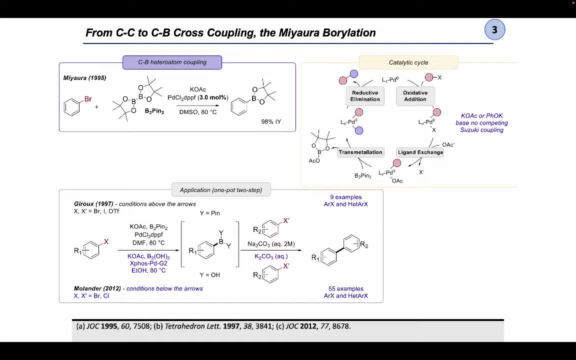 by Maiore Even today. bisphenicylato-d-boron, bis-diphenyl-phosphine-ferro-C and dichloro-palladium and potassium acetate are a smart choice for your first borrelation in the lab. 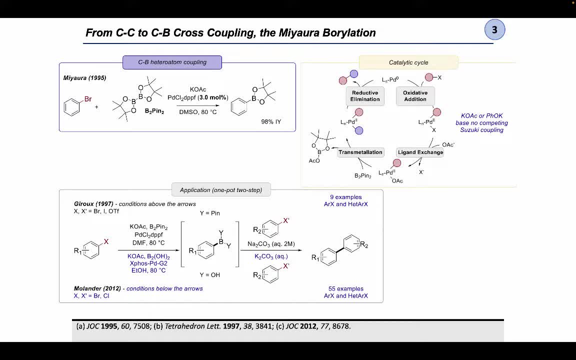 The use of a mild base instead of a strong base is very important, since it prevents a strong base. further Suzuki coupling of the aryl-boronate ester product, The Miara borrelation, is an attractive route to synthesize borrelated compounds under mild. 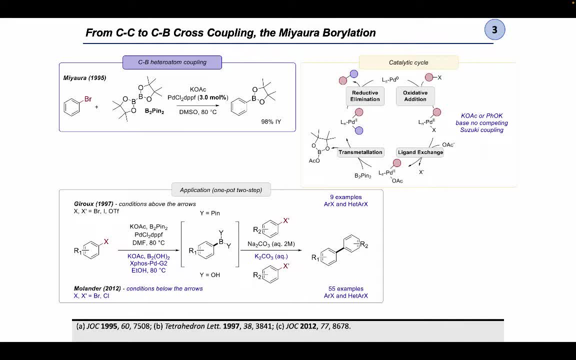 conditions, starting from readily available materials. Borrelation and Suzuki-Maillard cross-coupling have been combined in a one-pot, two-step procedure, for example early on by Giroud and more recently by the Molander Group. After completion of the Maillard borrelation, the Suzuki coupling is feasible simply by. 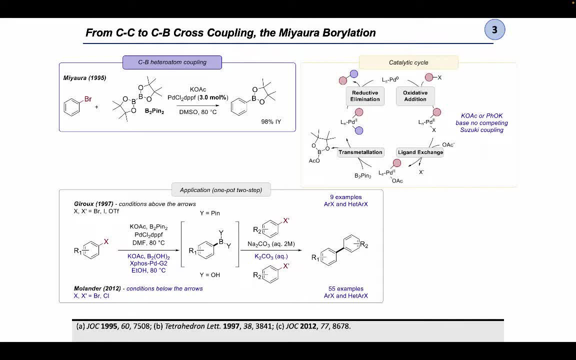 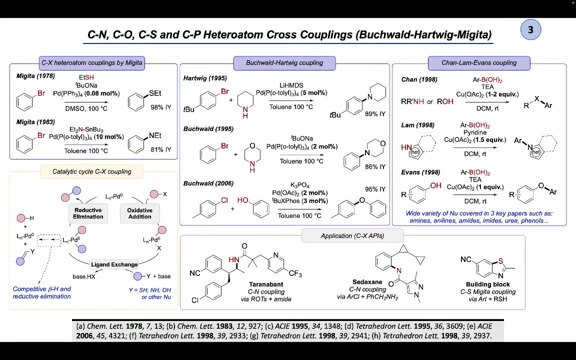 the addition of a second aryl halide and a strong base without in-situ isolation of the boronate. Cross-coupling towards carbon-heteratome bonds with well-known nucleophiles such as thyls amines and alcohols was early on studied by Migita. 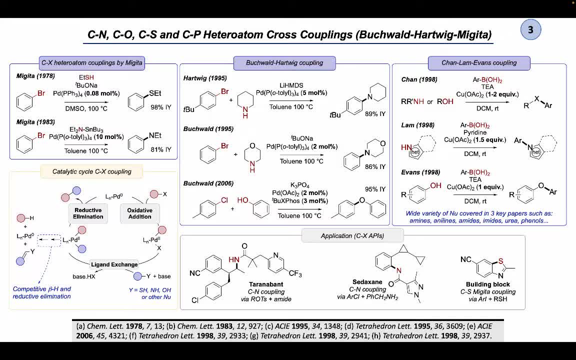 For example, already in 1978 he described the formation of a carbon-sulfur bond with catalytic amounts of palladium. Further studies were conducted by the group of Migita, Miyahashi and Beletskaya, and others as well. 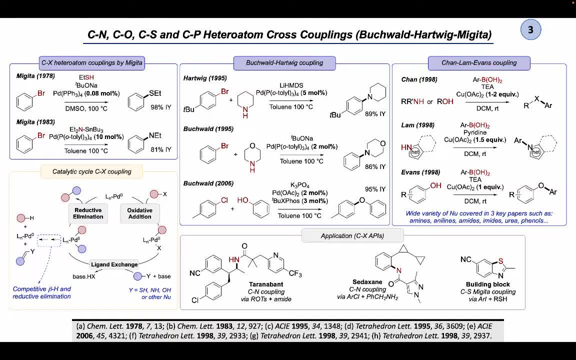 Another important contribution, also from the group of Migita and co-workers, was reported in 1983, where he described the first carbon-nitrogen-palladium-catalyzed bond formation. In 1995, both Buchwald and Hertwig improved the pioneering work of Migita by replacing 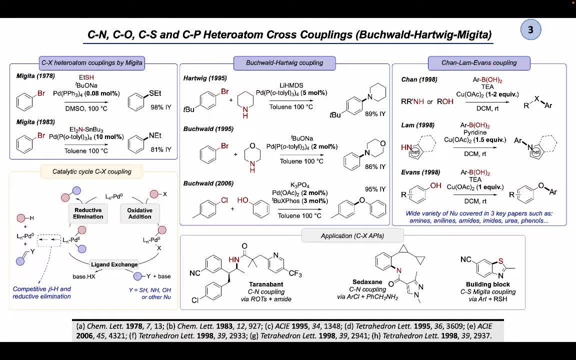 the amido-thin reagent by an amine and a strong base. The protocols developed by Buchwald and Hertwig were compatible with a broad variety of secondary amines and avoided the water-sensitive and toxic amino acids. Both protocols were quickly adapted by the scientific community. 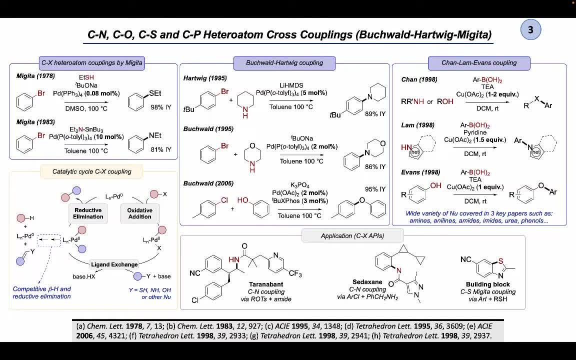 Buchwald, Hertwig and other groups further improved amination and improved or expanded the coupling to other nucleophiles, For example. Buchwald and co-workers also reported the mild palladium-catalyzed carbon-oxygen formation of diaryl-ethers in 2006.. The Chan-Lam-Evans coupling should also be mentioned, since it is complementary to the Buchwald-Hertwig coupling. The cross-coupling of the diaryl-ethers and the diaryl-ethers was also reported in 2006.. In 2006, the diaryl-ethers and the diaryl-ethers were combined. In 2006, the diaryl-ethers and the diaryl-ethers were combined. In 2006, the diaryl-ethers and the diaryl-ethers were combined. 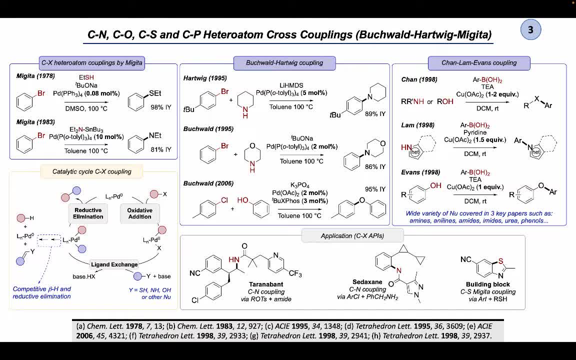 In 2005,, the duodenum ether and the diaryl-digest hybrid happened while the laomethium ether was expanded. This signified the enhancement of nuclear informations in the diaryl-ahers and duodenum ether. Stalkium copper also formediscal events in 1926.. 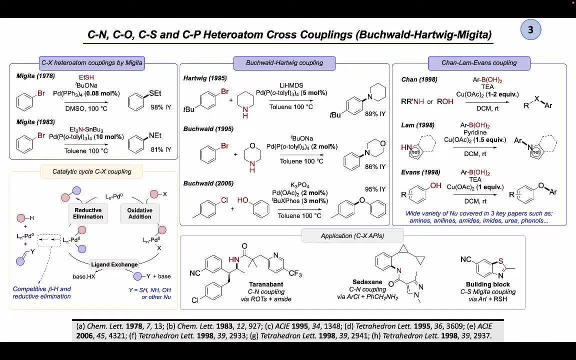 The duodenum ether states. no элемents should be concerned with coalescence. Same thing…. Searching for the chlorgyne certification gene or influenza alone results in a very interesting transformation…. Open supply chains were created in EP in 2002.. 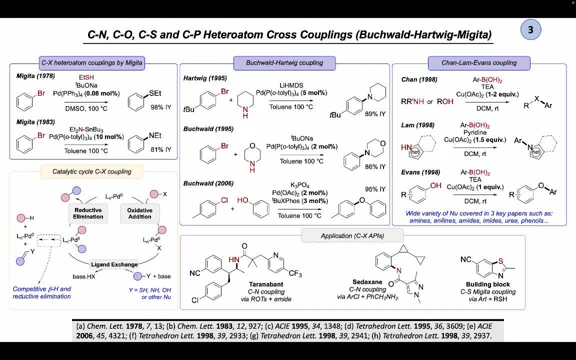 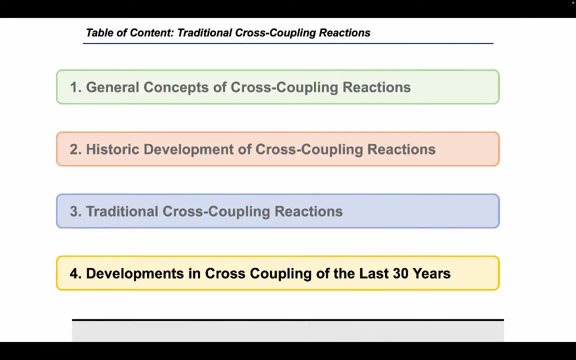 10. Thus it also follows a different mechanism compared to the palladium-catalyzed Buchwald-Hartwig coupling. At this point we have only focused on the narrative of the development of conceptually new reactivity cross-couplings. 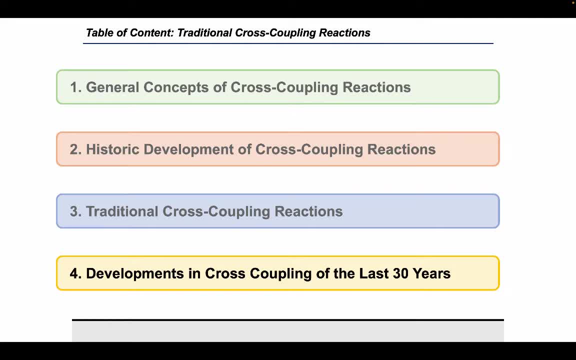 Of course, the deep understanding and continuous fine-tuning with the aim of increasing functional group compatibility, thus increasing applicability, was and is still ongoing. at this point, The importance of these modifications and manipulations should not be underestimated, since they made it possible to begin employing carbon-carbon coupling chemistry in the synthesis of biological important molecules, even on large scale. 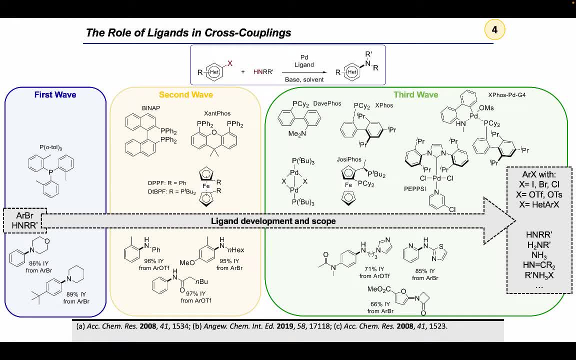 The detailed work by both Buchwald and Hartwig on the mechanism and the development of improved catalytic systems for deamination is an excellent example to illustrate the potential impact of fine-tuning in cross-coupling. Thanks to these developments, the mechanism is now in place. 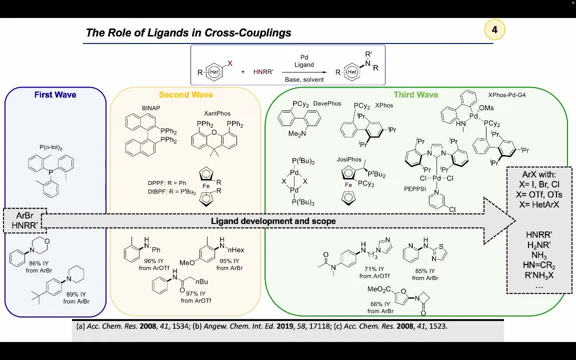 The Buchwald-Hartwig amination has become a fundamental tool in organic synthesis for the formation of carbon-nitrogen bombs. The initial report previously discussed relied on the orthotolylphosphine ligand. This allowed the amination of aliphatic and cyclic secondary amine nucleophiles with aryl bromides or iodides. 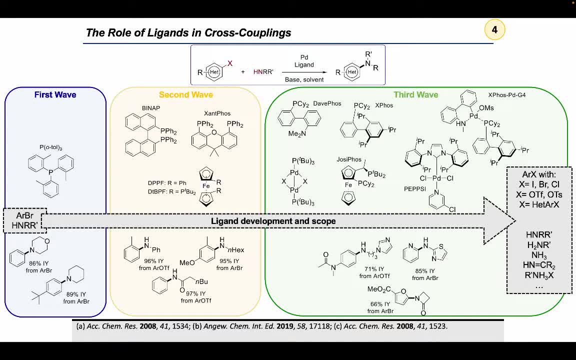 Less reactive electrophiles and primary amines were not feasible. Both groups introduced a second wave of ligands based on aromatic biphosphine ligands. The second wave of ligands was the aryl bromide ligand. The rationale was to improve performance by having the bidentate coordination of phosphine to the metal center, thus favoring reductive elimination over the competing beta-hydride elimination. 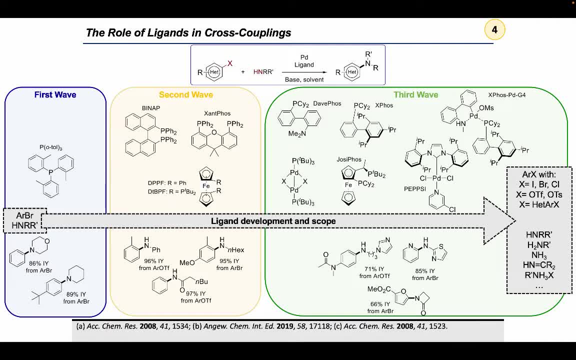 Both groups independently reported BINAP and DPPF as ligand. The yield was improved and both the electrophilic and nucleophilic partners' scope was expanded. For example, aryl triflates or alkyl bromides or primary amines were successfully cross-coupled. 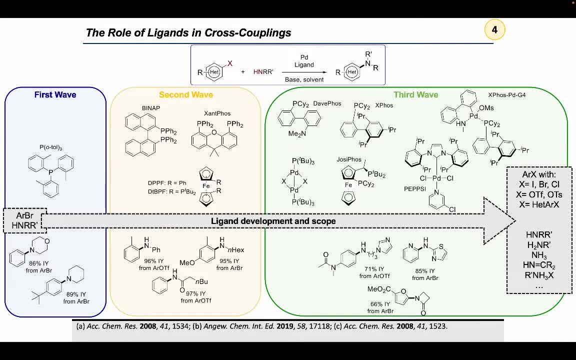 Further building on this rationale, even more steroid bulk- The scope was introduced, resulting in, for example, DTPPF and pop-type ligands such as Xanthos. With these ligands, the scope was again expanded to include, for example, aryl chlorides and also weaker nucleophiles such as anilines and amides. for the first time, 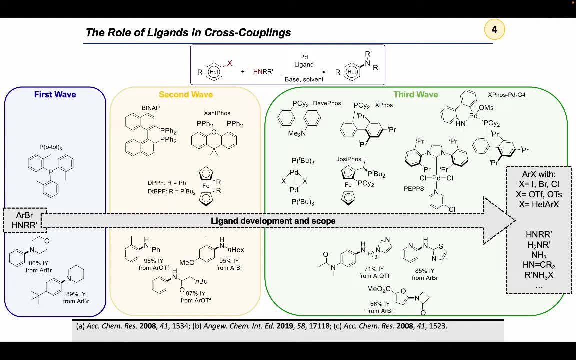 In a third wave both switched to sterically hindered monophosphine ligands. The rationale was to increase electron density around the metal center, thus accelerating the slow oxidative addition step and secondly keeping the reductive elimination. The results were very fast by having the steric hindrance present. 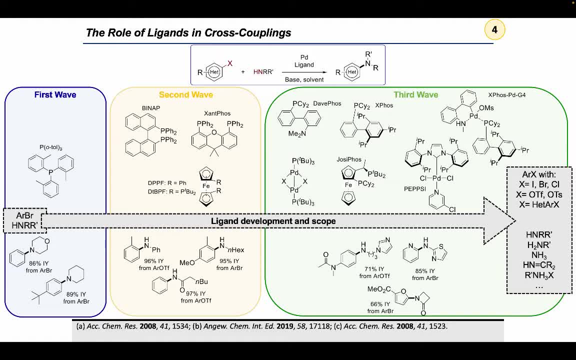 In the lab of Brugwald, a series of biaryl phosphines such as DEFOS and XFOS were developed, while Hartwig investigated trialkyl phosphine and JolciFOS-type ligands. Both series improved catalytic efficiency allowed the reaction under milder conditions. 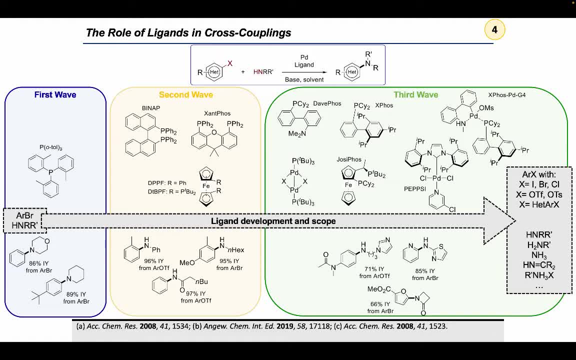 and expanded coupling partners' scope to, for example, aryl chlorides and various pseudohalides, coupling with heteroaryl halides and selective emanation with ammonia. In the previous slide and throughout this presentation, pseudohalides were already shown or mentioned. 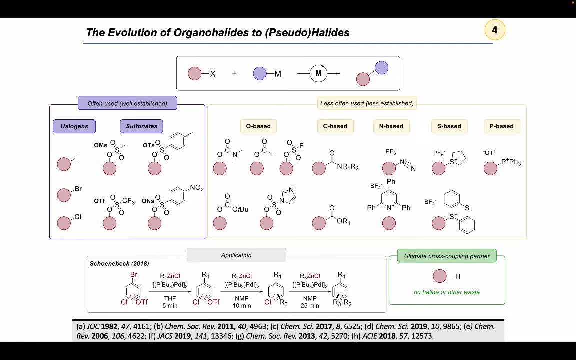 Historically, the initial focus in cross-coupling was on finding new nucleophilic partners, so the organohalide, mostly iodide or bromide, remained the same for many years. The first pseudohalide reported in cross-coupling was hiranyl, acetate by Negishi in 1982.. 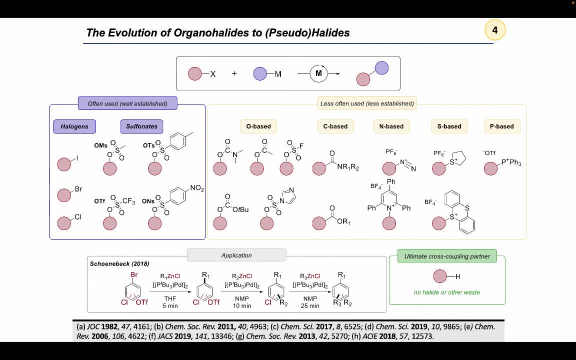 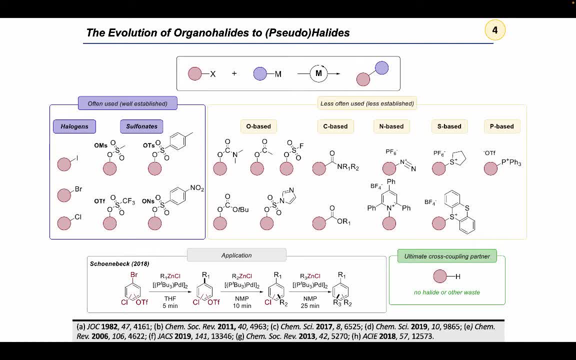 be said that this selectivity is not general and depends on substrate, catalyst and reaction conditions. Of course, the ultimate goal would be to selectively achieve CH functionalization and if possible in complex molecules. This would be the most efficient strategy, but this field is not discussed today. 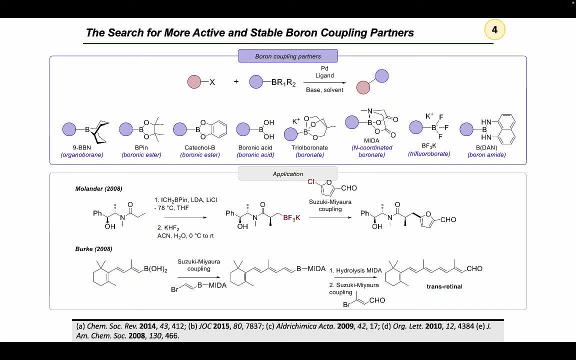 The most popular of cross-couplings in organic synthesis has always been and remains the Suzuki-Myaure coupling, Since boronic species are essential in this coupling. alternative boron species have been investigated thoroughly, Initially alkyl needle, boranes and catechol. 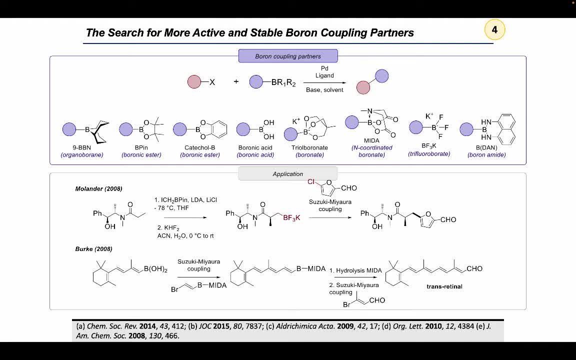 boronic esters were used. however, by now, a wide variety of boronic species are available. Some of the most popular ones are shown, yet more are out there. Reason for the development of new boronic species are easy preparation, increased stability. 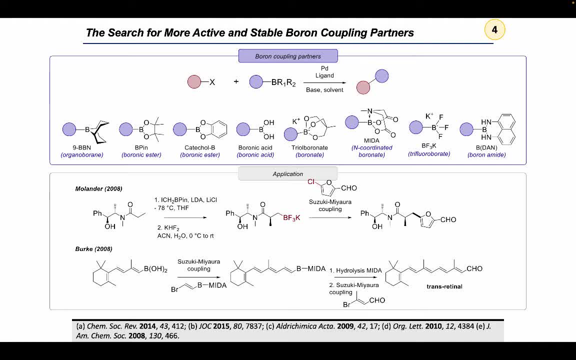 easy-to-handle solid boron analogues, development of efficient synthetic strategies, boron species stable towards silicon, and high-density synthesis. More details about the pro and cons of each can be found in the references below. Trifluoroborate salts and mida-boronates are the most developed systems, For example as: 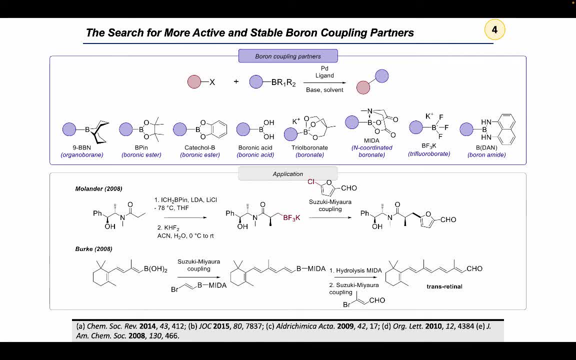 reported by Molender and co-workers, stable trifluoroborate salts were prepared and subsequently derivatized by cross-coupling with various aryl chlorides. Secondly, iterative cross-coupling strategy using mida-boronates has also been developed. 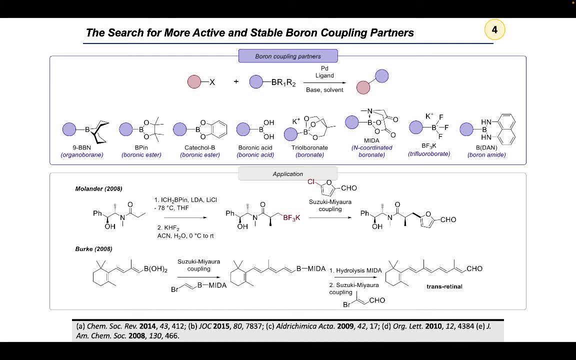 For example in the synthesis of polyene natural products such as retinol. the synthetic approach is only feasible because mida is stable under certain Suzuki-Miyare conditions but can be deprotected rapidly to unmask another boronic acid reactive group. 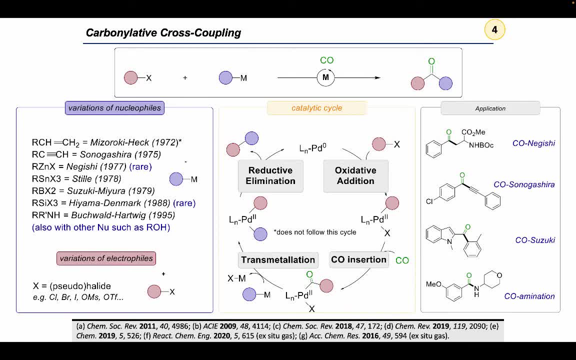 Carbonolative variations of almost all well-known cross-couplings have been reported by different groups. CO insertion is a fast process so it can be easily incorporated in the catalytic cycle. Carbonolative reactions are an efficient methodology for the synthesis of carbonyl-containing compounds. 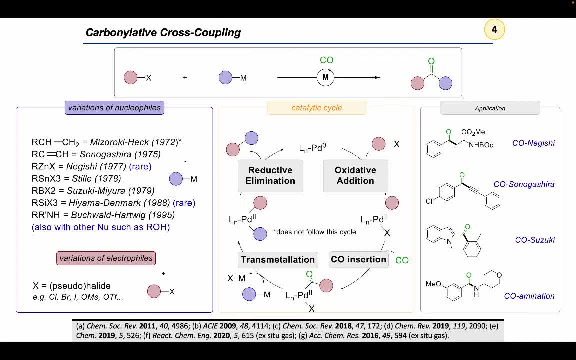 Mostly ketones are formed, but also, for example, amides, esters and alkenones are feasible. Of course, one should be careful when working with a toxic gas as carbon monoxide. Despite this, solid CO precursor compounds and commercially available simple lab equipment are out there. 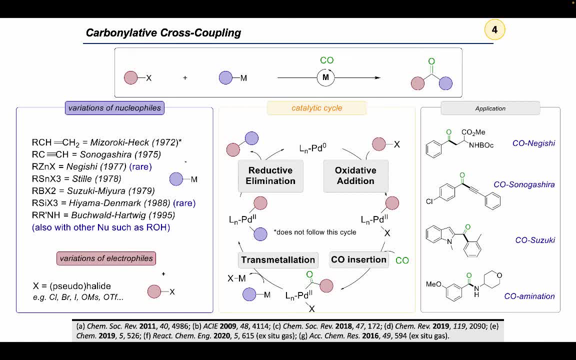 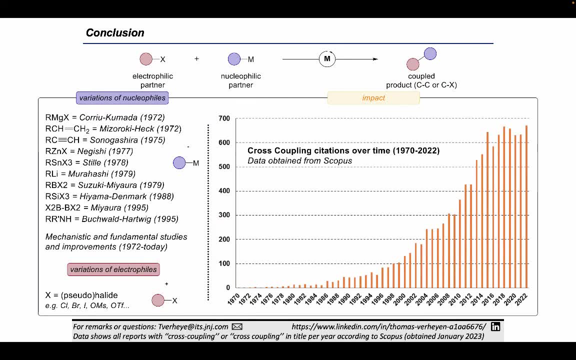 thus omitting the necessity of specializing in the process. Thank you. Some of the examples presented today have received more attention than others. Nonetheless, all the transformation and following mechanistic and optimization research have played an important role in the development of cross-coupling. This effort has pushed the boundaries of possibilities. 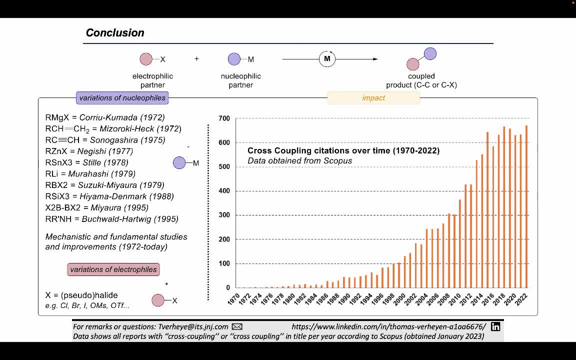 and led to the current state of the field. The field continues to receive attention from both the academic and industrial community. I personally also look forward to the next developments in the field. So what's next? Cross-coupling is still evolving, by, for example, looking into the merger of: 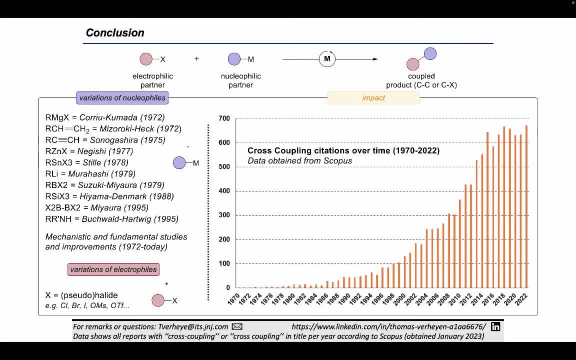 cross-coupling with other fields such as photoredox, electrochemistry, high throughput screening and artificial intelligence. By looking at new types of related reactions, such as cross-electrophile coupling. by looking at novel, easy, accessible pseudo-highlights. by looking at the latest. 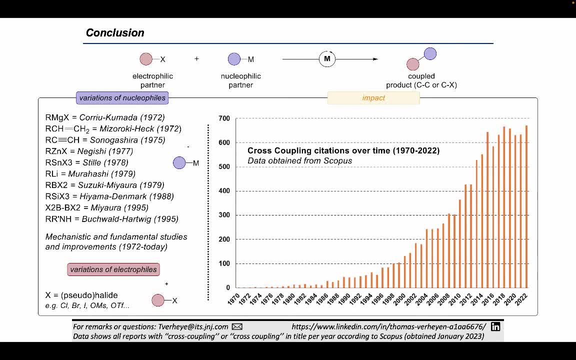 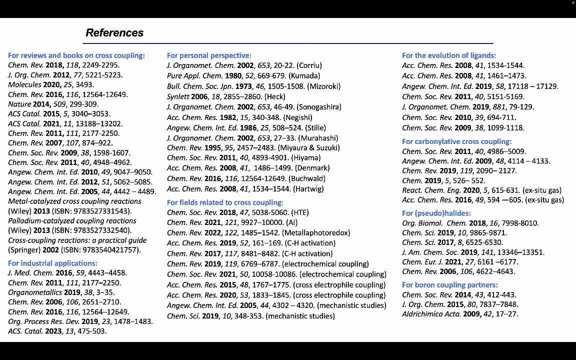 analytical techniques to further understand the mechanistic aspects, or by generating and theoretically mapping new and own catalystic systems. and, of course, also CEH activation remains an area of interest. I would like to close today's episode by mentioning that only the highlights were touched, however. 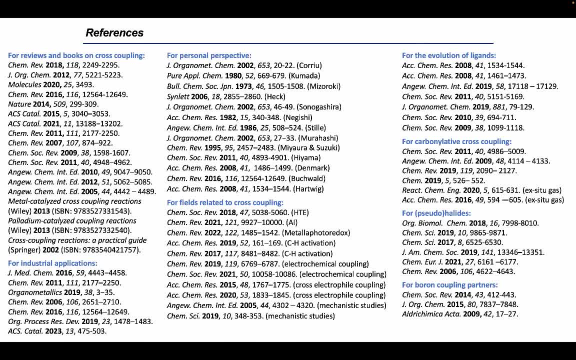 many other relevant contributions were made. For those who want to learn more. on this slide you can find some excellent literature references which were used to construct this episode. I might have also mispronounced some of the names, for which I apologize. Finally, 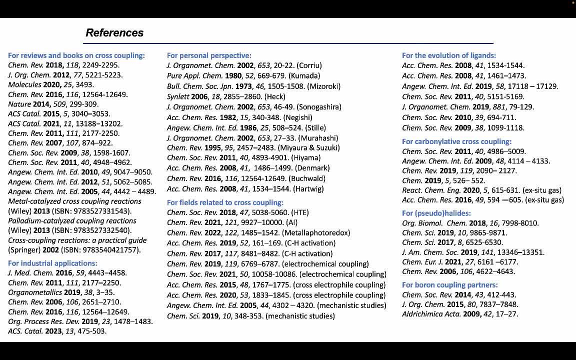 thank you for your attention And feel free to reach out to either me or Matt in case of any questions. If you're interested in more episodes in the future, to cover some of the recent trends, for example, you can also let us know.